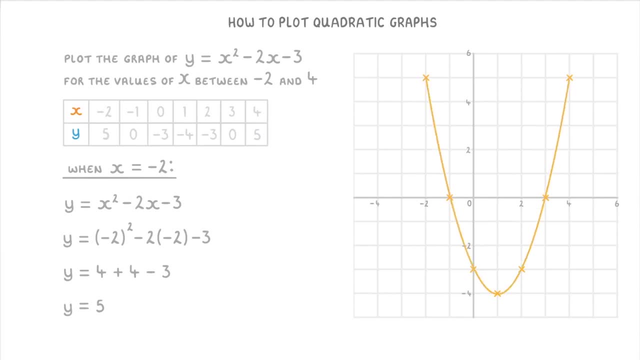 you can join them all up with a smooth curve. The fact that your curve is smooth is actually really important. If you instead were to use straight lines like this, then you wouldn't get the marks. Another important point is: whenever you do these questions, it's always good to check if your graph looks right, For 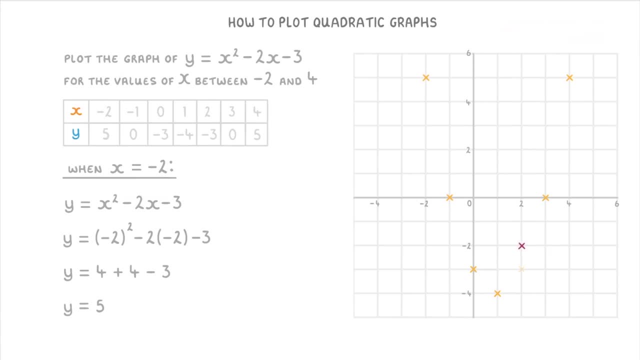 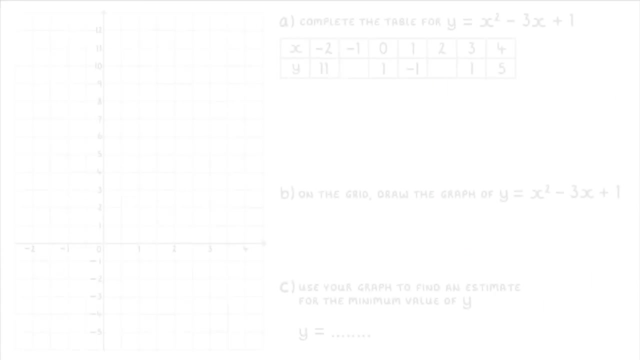 example, if one of our coordinates had been over here, then when you joined all of your points up, you would get this little bump in your line, which is obviously wrong, and so you would know that you need to double check your workings for this point. 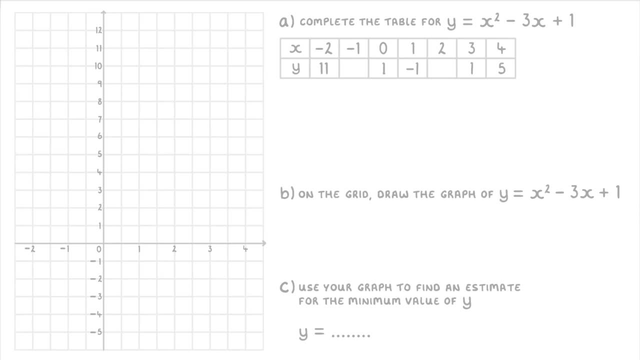 Let's now have a go at a real exam question. Give the video a pause if you want to have a try. So basically, this question has been split up into three parts. In the first part, we need to use the equation to complete the table which they've already started for us. Then 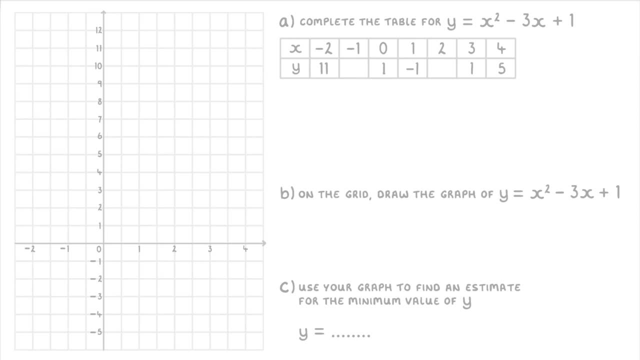 for part b, we have to draw the graph, which we can do by plotting all of the points and then joining them all up. And finally, for part c, we need to use the graph to find an estimate for the minimum value of y, which we haven't covered yet, but is just the. 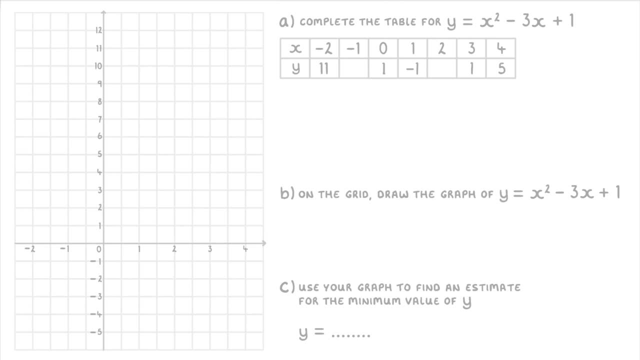 lowest possible value. So, starting with part a, the first thing we need to do is find out what y will be when x is minus 1.. So we just plug minus 1 into the equation, which gives us y equals minus 1, squared minus 3 times minus 1 plus 1, which means that y equals 5.. Then we need to do: 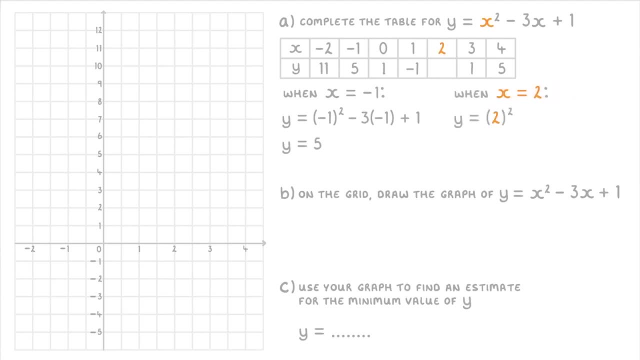 the same thing for when x equals 2.. So y will equal 2 squared minus 1 squared minus 1 squared 2 squared minus 3 times 2 plus 1, which is minus 1 this time. Now that we've completed the table, we can move onto part b, Before we can actually draw. 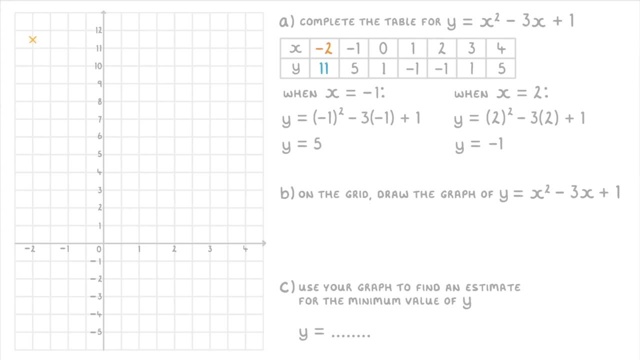 a graph, though we need to plot all of our points. So, minus 2, 11,, minus 1, 5,, zero, 1, 1 minus 1,, 2 minus 1,, 3, 1 and 4, 5.. And then we can join them up with a knight's structure.